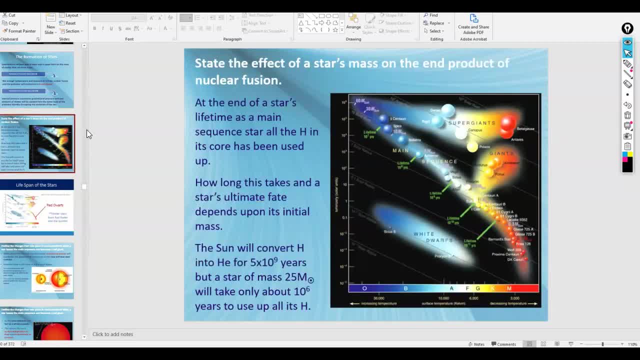 that all the stuff is going to get like blown out. Okay, we talked about main sequence stars, which a main sequence star basically lies on that middle diagonal band on the HR diagram, and a main sequence star is one that is primarily fusing hydrogen into helium. 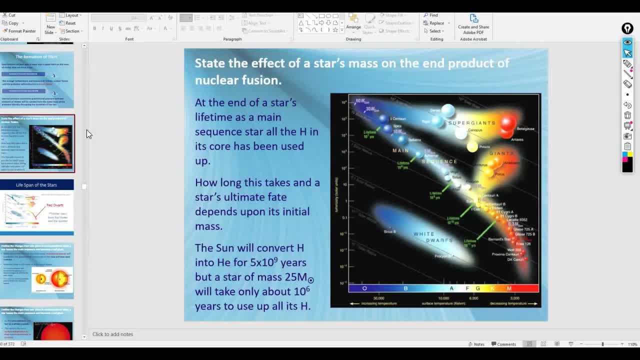 Now, at some point at the end of a star's lifetime or close to the end of a star's lifetime as a main sequence star, what can happen is all of the hydrogen in that core can get used up And how long that takes. 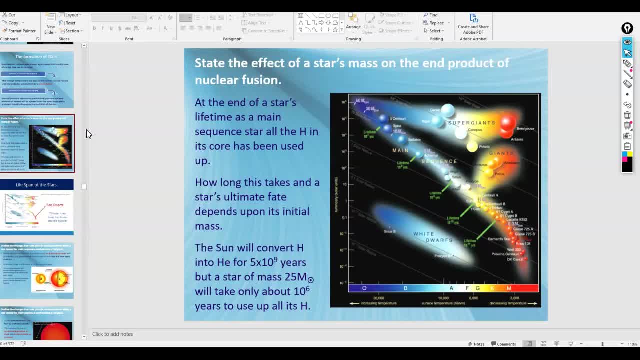 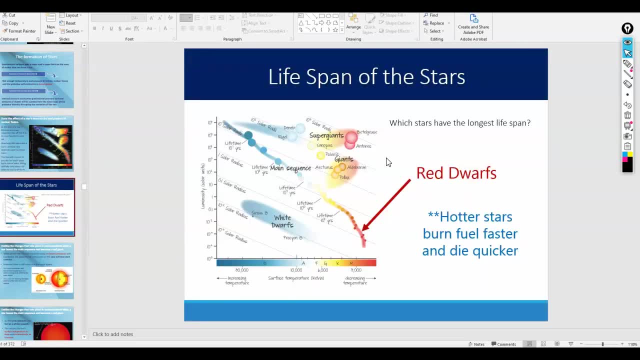 Like a time, As we talked about in the last video, it kind of depends on how much mass the star had to begin with. Bigger stars tend to not live as long as smaller stars. Okay, and so, for example, here you can see on this chart that the stars that have the longest lifespan are going to be Reddorfs. 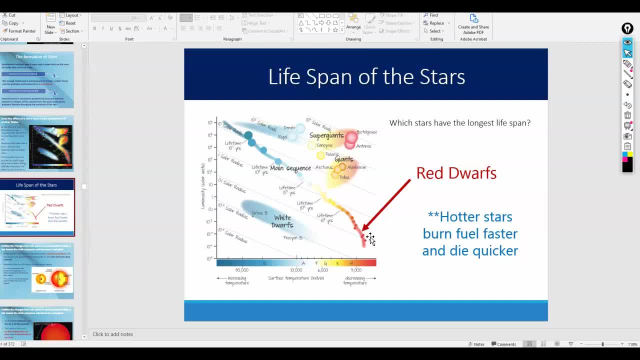 Those are stars that initially formed. they had enough mass to form a star, but not enough mass to be super big or super hot, And so they're relatively cold stars compared to other stars, which means that they last longer, Okay, whereas you could have blue giants that only last like a couple million years. 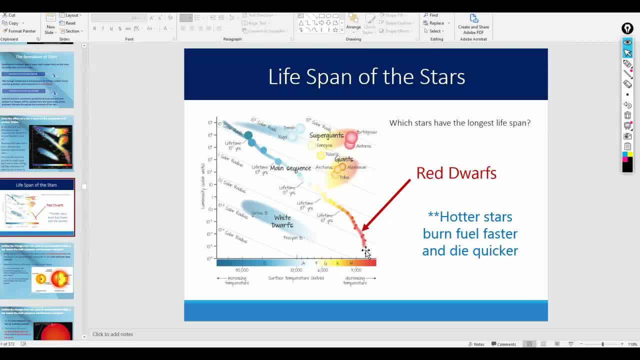 You could have Reddorfs, that last. you know hundreds of billions, if not trillions of years. Our star is about, you know, four to five billion years old, And so our star is kind of like an average star. 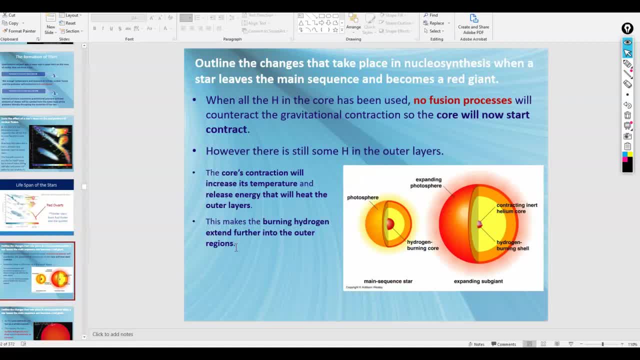 Anyway. so what can happen at the end of a star's lifetime, as a main sequence star, is that all of the hydrogen gets used up, which basically means that, at least temporarily, no fuses. Okay, and so in a normal star you have this equilibrium between the inward gravitational pressure because of all the mass. 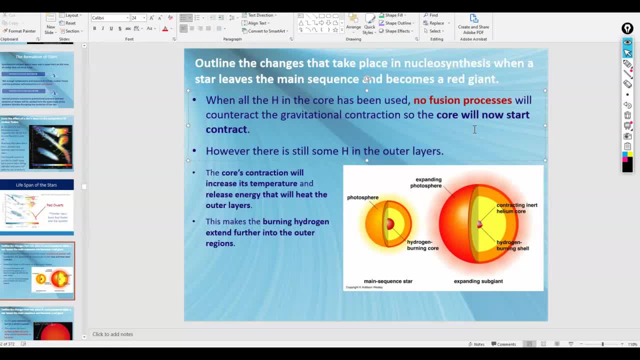 and the outward radiation pressure from all of the fusion. And so if the hydrogen gets used up and the fusion stops, then there's nothing to counteract the gravitational force, And so the core is going to start to contract and get smaller. However, when that happens, when the mass gets close together and it gets dense- 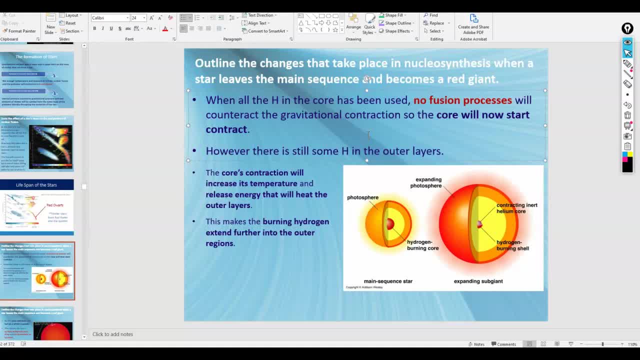 the temperature inside the core is also going to get hotter, And what can potentially happen is you still have some hydrogen on the outer layers of the star And so, as the core contracts, the temperature of the core is going to go back up, And that could possibly ignite further fusion reactions, further fusion of hydrogen. 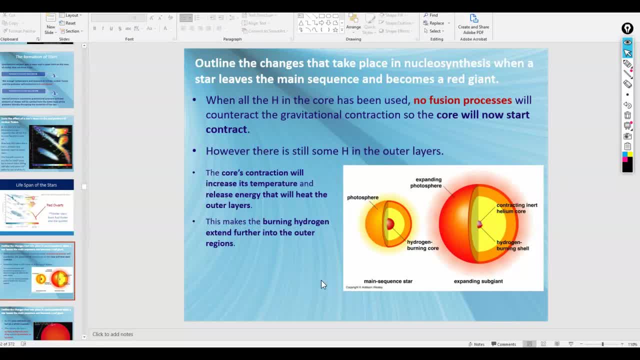 But it's also possible that the contracting core can actually create temperatures so high that, rather than fusing hydrogen into helium, you can actually create a fusion of hydrogen into helium. You can actually fuse helium into heavier elements like carbon or oxygen or heavier elements like that. 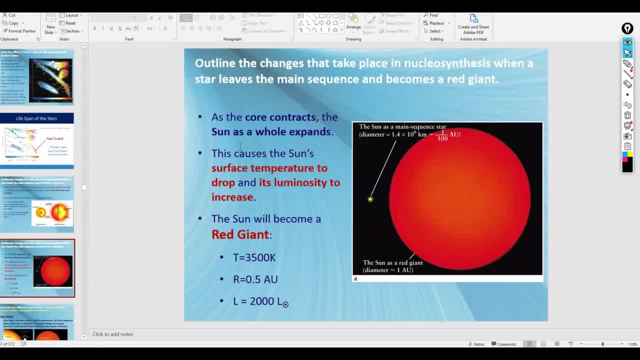 Okay, and so that's also a possibility. Now for our sun. what's going to happen is as the core contracts, and it's giving off more heat. the sun as a whole is going to expand And it's going to become what's known as a red giant. 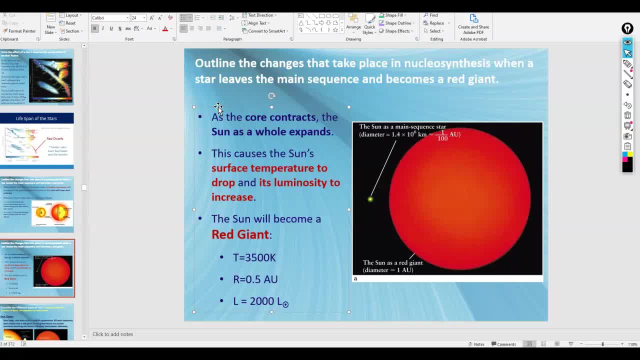 And the size of the sun is actually going to get out to about where the Earth is located, And so it's very possible that Mercury, Venus and maybe even the Earth are going to get swallowed up by the red giant sun, And because, because the sun is expanding, the surface temperature is going to drop. 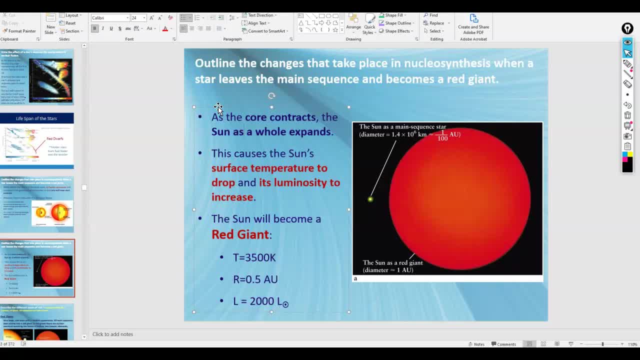 And so because it's not as hot. that's why it's going to go from being like a yellow star to a red star, But the luminosity is going to increase because, even though it's colder, it's also like way bigger, because it's going to be a red giant. 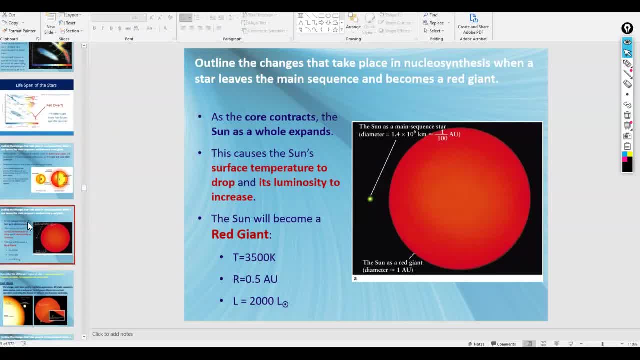 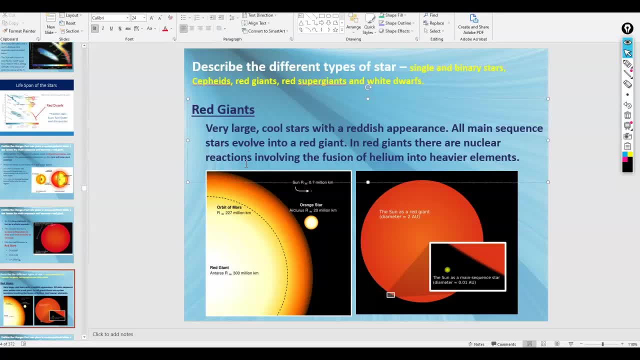 And so at some point, probably in a couple billion years, this is going to happen to our sun. It's going to To enter its red giant stage. And again, red giants are very big, relatively cool stars with a reddish appearance. 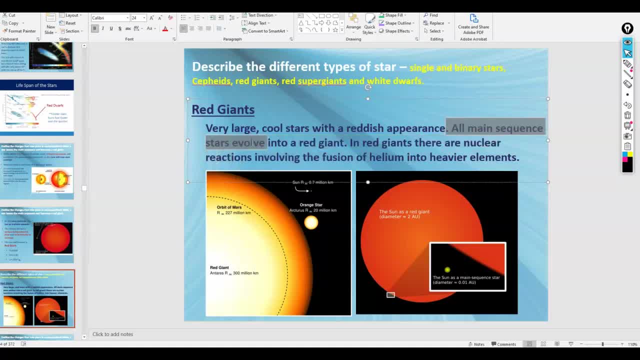 As you can see here In the notes, all main sequencers at some point evolve into a red giant, And in a red giant there are nuclear reactions involving the fusion of helium into heavier elements, And so this process that I just described before- fusion, stopping gravity, causing the core to contract. 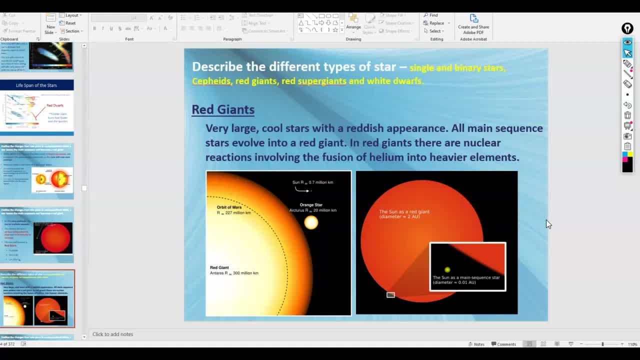 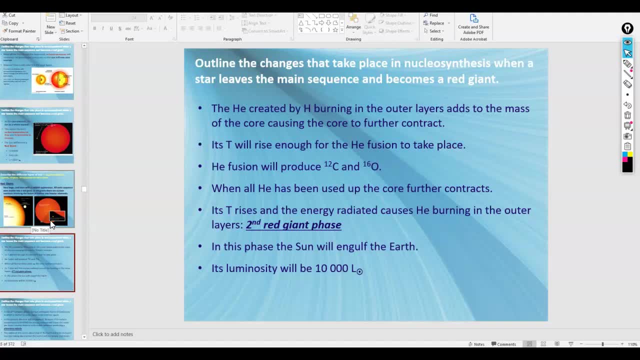 leading to higher temperatures, leading to possibly more fusion. If the star is big enough, that can actually keep happening and keep happening And at some point you could run out of helium, And when you run out of helium the core could contract further and cause higher temperatures. 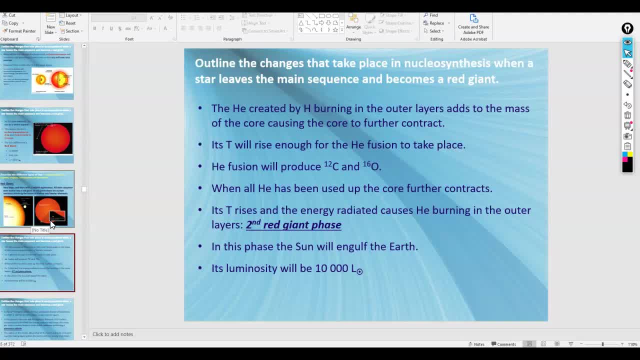 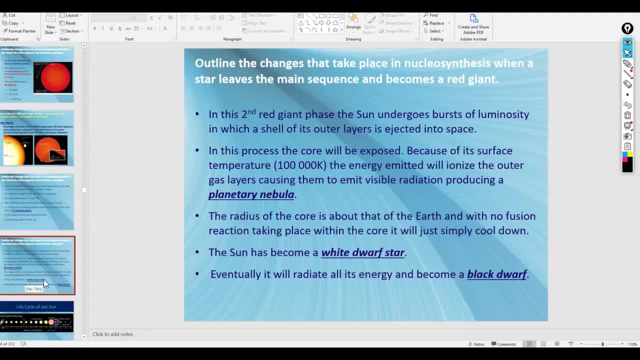 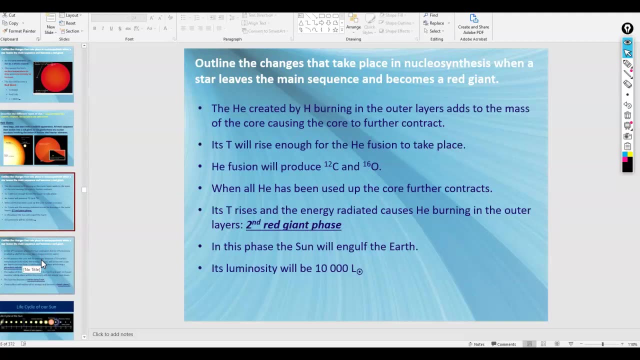 And then you could start fusing carbon and oxygen and neon and magnesium and even heavier elements, And so the number of elements you get kind of just depends on the mass of the star. OK, now, At some point, though, this whole process is going to stop. 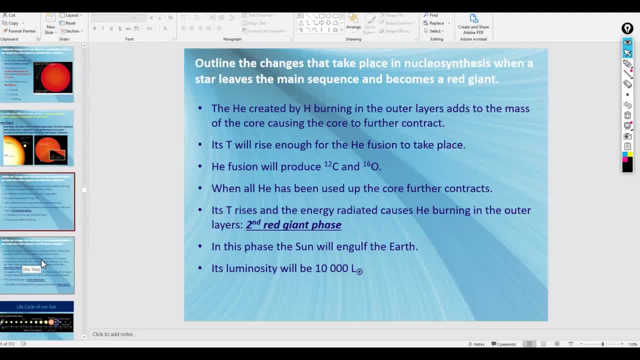 At some point the core is going to contract and the temperatures are going to go up, but it's not going to go up enough to cause additional fusion, And so, in the end, gravity is basically going to win. Now, when that happens, 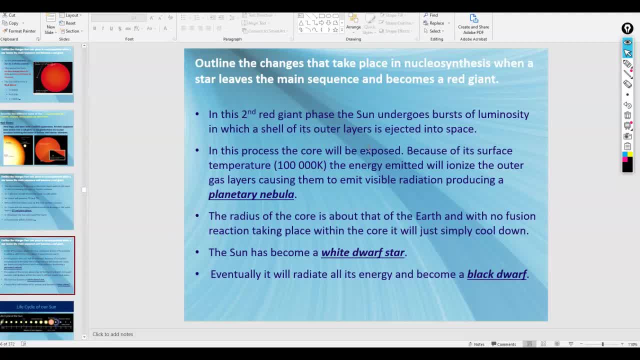 Basically, The way this works is the sun. This is like imagine that the very end of our son's lifetime. This is what's going to happen. OK, so you have the red giant. OK, In the very center of the red giant you have the core of the star. 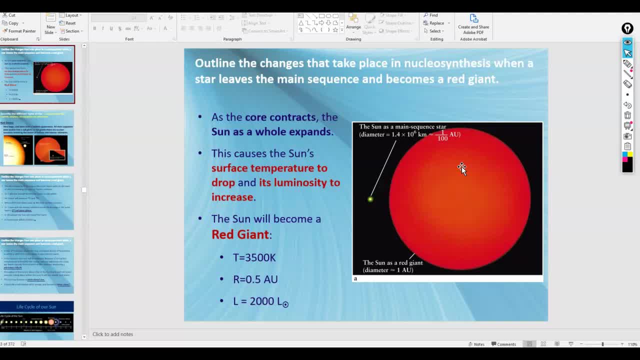 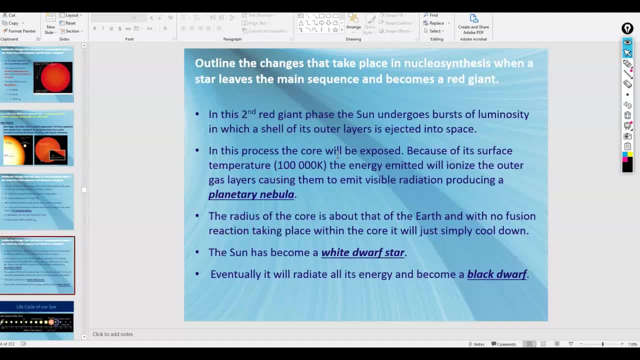 OK, At the end of our son's lifetime, what's going to happen is Is the outer layer is going to kind of float off into space and it's going to produce what's called a planetary nebula. And so this is kind of like like the outside of the, the, our sun, just kind of like floating off into space. 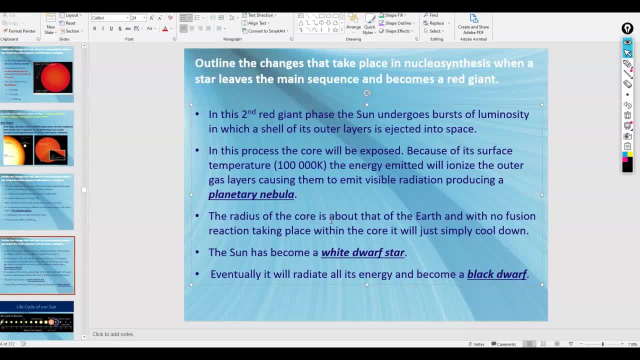 You get this planetary nebula. This is the planetary nebula. Now the core that has no more fusion happening, is basically done. OK, it's dead, There's no more fusion happening. It's really hot because it's been fusioning for billions of years, but it's basically going to end up about the size of Earth. 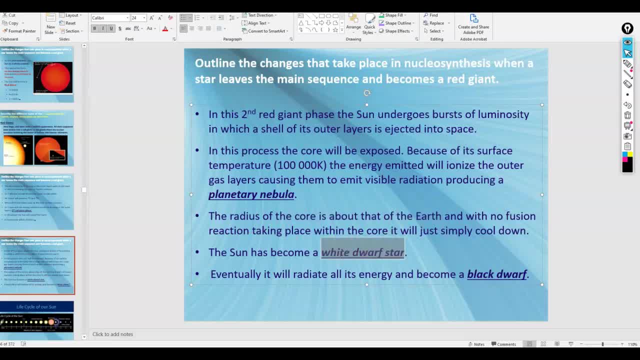 There's not going to be any fusion happening. This is what's called a white door star. OK, a white dwarf and a brown dwarf and a red dwarf are not all the same thing. They're not all like different colors of the same thing. 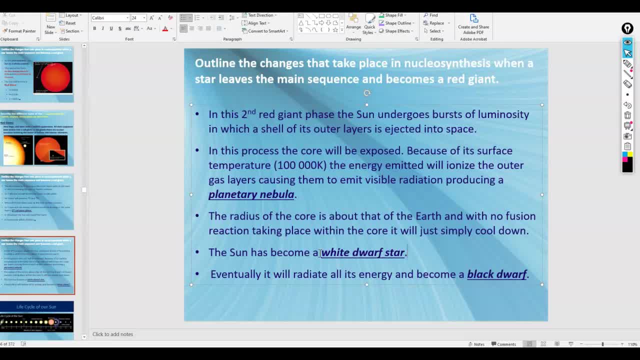 A brown dwarf is a star that never even got going. A red dwarf is, like it's, a main sequence star that just happens to be small and red. A white dwarf is the end stage of a star that's around the size of our sun. 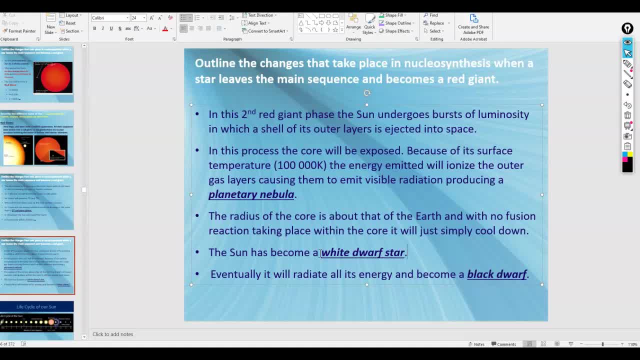 A white dwarf star is not even really a star because there's no fusion happening. It's basically just the, the really hot core of a star. that used to be a lot And eventually what's going to happen is because there's no more fusion happening, there's no more new heat or new energy being produced. 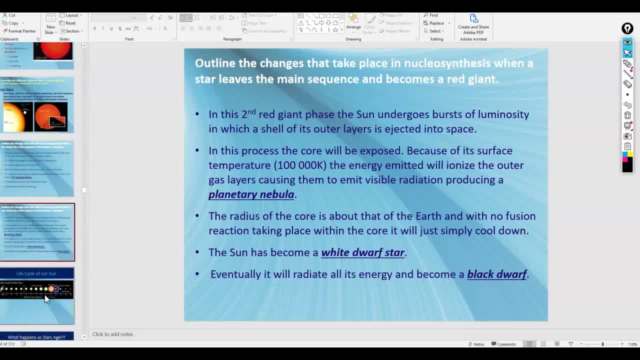 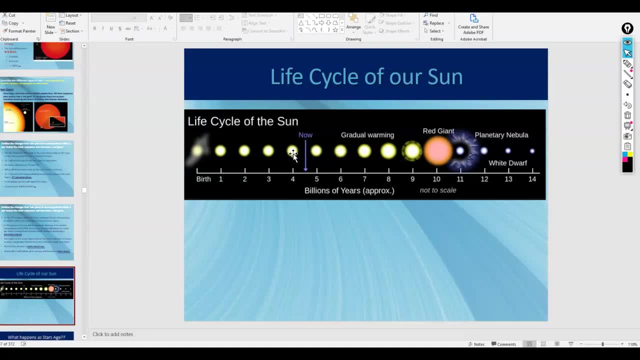 Eventually it's just going to cool down and be dead and that's going to be the end of our sun. So here you can kind of see the life cycle of our sun. We're kind of like here in the timeline, but eventually it's going to grow into a red giant. 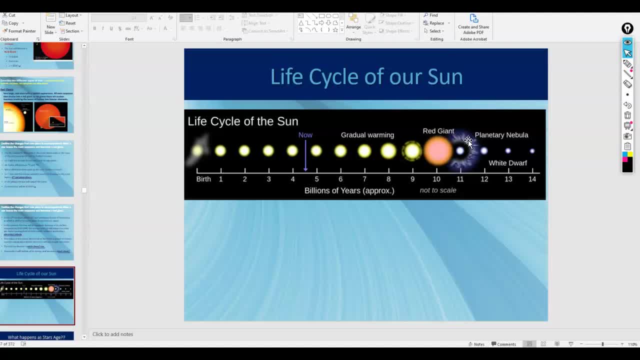 The outer shell is going to kind of puff off into space, form that planetary nebula that you can see, And the core that gets left behind is going to be about the size of Earth, And that's the white dwarf. OK, and so that is going to be what's going to happen. 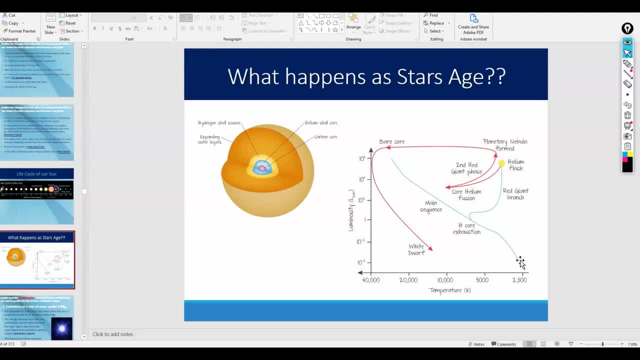 It's going to happen to our sun And you can imagine- I said this in the last video, if you imagine- like the HR diagram, a star's position on the HR diagram is not fixed And so over time, what's going to happen is our sun is going to move around the HR diagram as it forms, you know, into red giant phase and its second red giant phase and the planetary nebula. 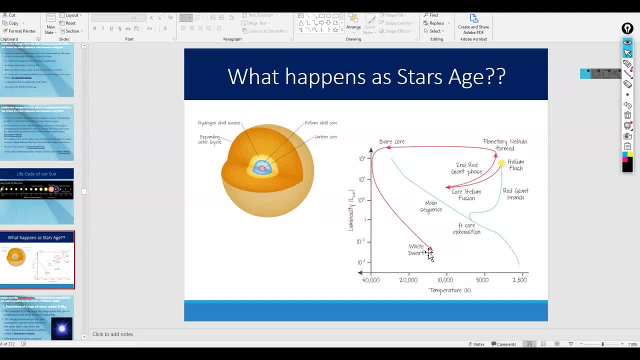 And then eventually it's going to end up as a white dwarf and it's going to be really hot but really small and low luminosity, OK, and so this is kind of going to be our sun's evolution on the HR diagram, And I said this before. but you can get layers of different elements in a star because once that hydrogen fuses into helium, when the core contracts and the temperatures go up, that helium can start fusing into carbon. 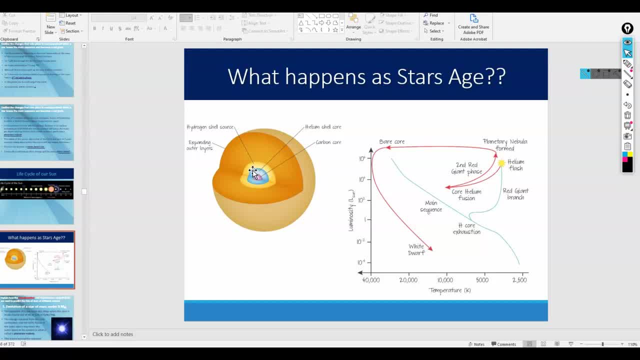 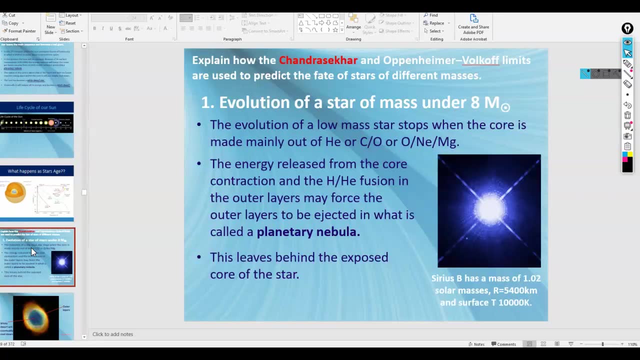 And so our sun is probably going to end up with, you know, some carbon in its core, maybe some heavier elements. I'm not sure exactly What elements are going to end up in our sun. but yeah, so that's basically the evolution of a star. that's relatively small. 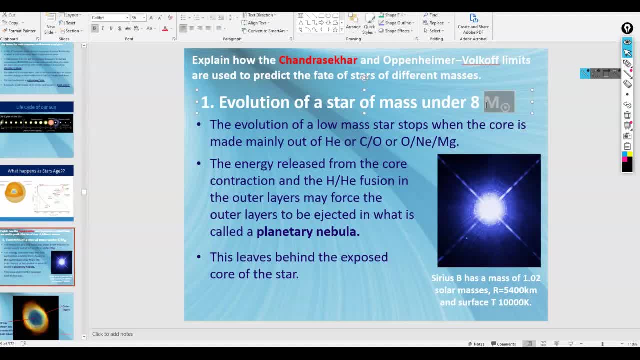 And what we say? the evolution of a star of mass less than eight solar masses. OK, so the evolution of low mass stars stops when the core is mainly consists of only helium, or maybe carbon and oxygen, maybe some oxygen, neon or magnesium. 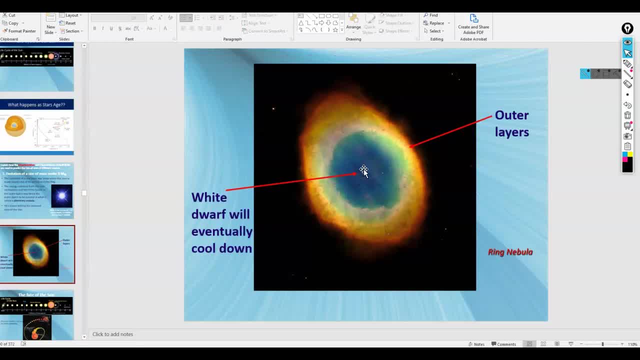 And we already talked about the planetary nebula. Here you can basically see like this outer part is like the outer shell of the red giant, just like puffing off into space. That is the planetary nebula. at the very center is the white dwarf that you can't even see because it's so small. 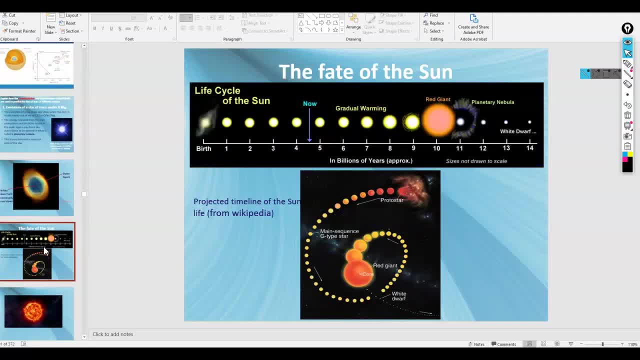 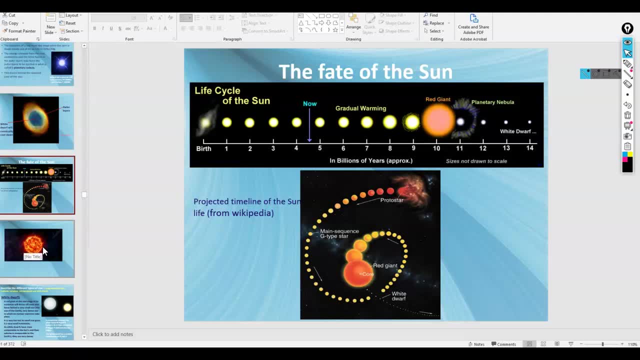 OK, so that's what's going to happen to our sun Now. it's possible you might have heard of a supernova, or you might have heard of like a black hole. Our sun is not going to do any of those things because it doesn't have enough mass. 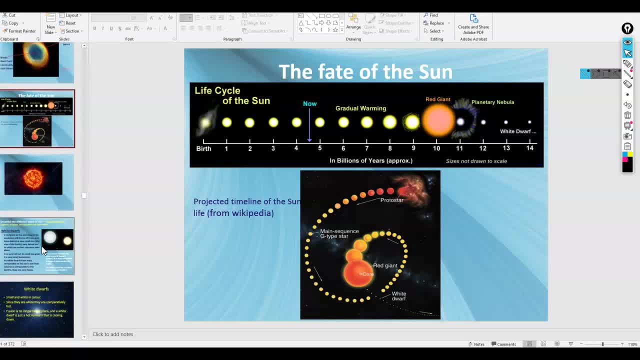 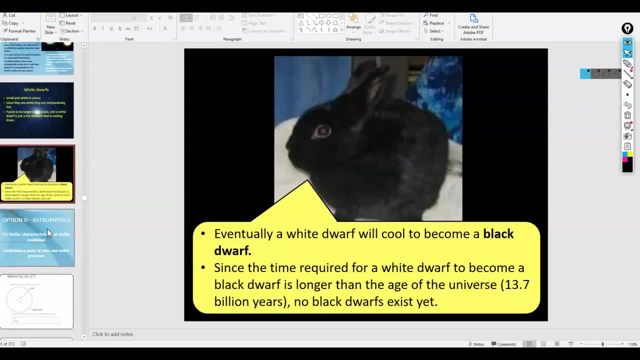 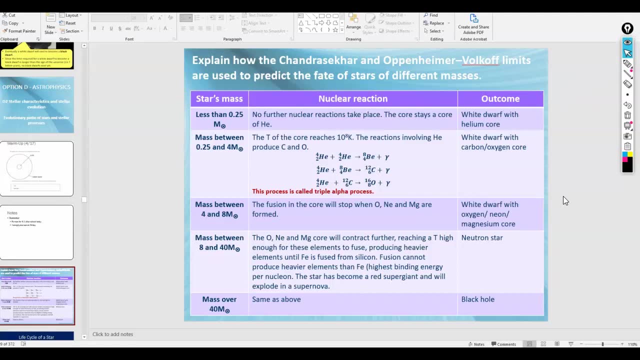 Our sun is going to. It's going to end up as a white dwarf, So Let's move on. And so so far, there's different outcomes for different stars. We've basically been talking about what's you know, our sun, which is like a normal, regular sized star, and our sun is going to end up as a white dwarf with a carbon-oxygen core based off of its mass. 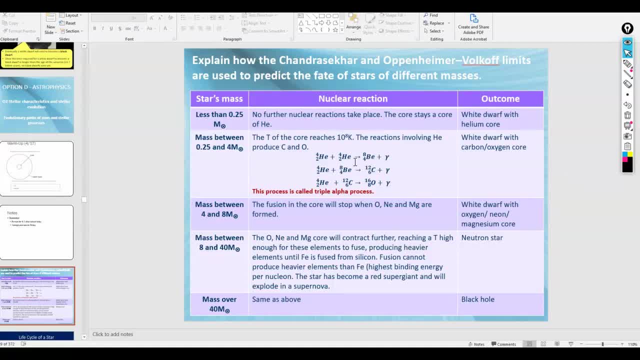 OK, now if you look at this chart, This chart kind of shows you like the different possible outcomes of a star based off of its mass. And so our sun has a mass of one solar mass, like by definition, And so our sun is going to fit into this like second row on this table. 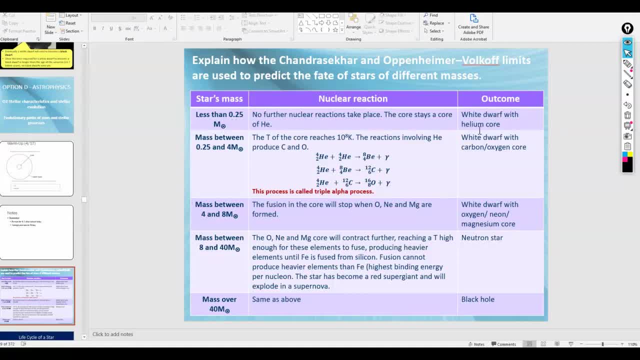 OK. stars that are smaller than 0.25 solar masses basically just end up with helium in its core. Stars that are slightly bigger than ours are going to maybe fuse higher elements like oxygen, neon or magnesium. Now what if you have? 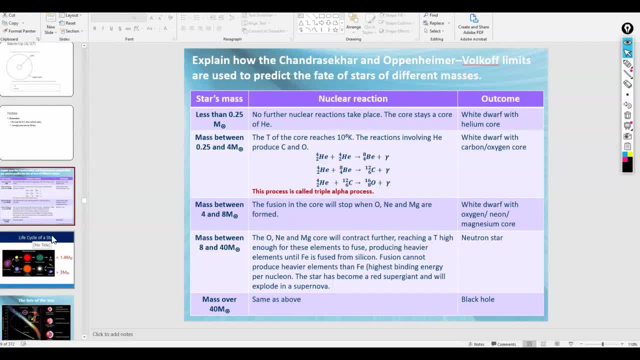 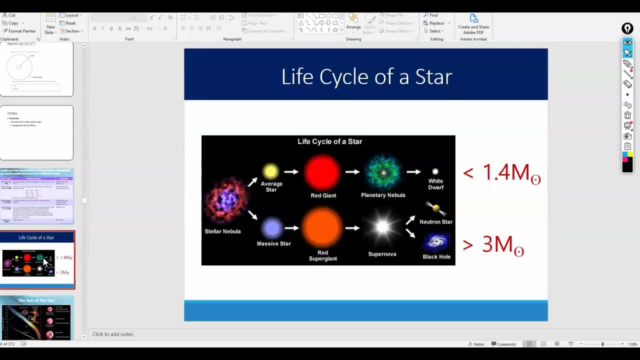 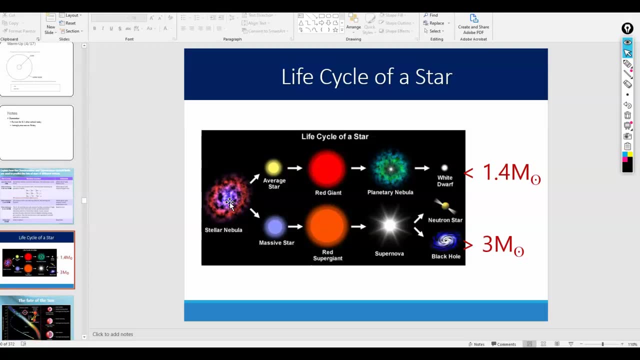 Bigger stars than eight solar masses. What's going to happen then? OK, so now things get interesting. If you have really really big stars, you can have other possibilities because of all the mass. OK, this chart right here kind of shows you the entire life cycle, starting from, starting from like a nebula and ending as either a white dwarf, neutron star or black hole. 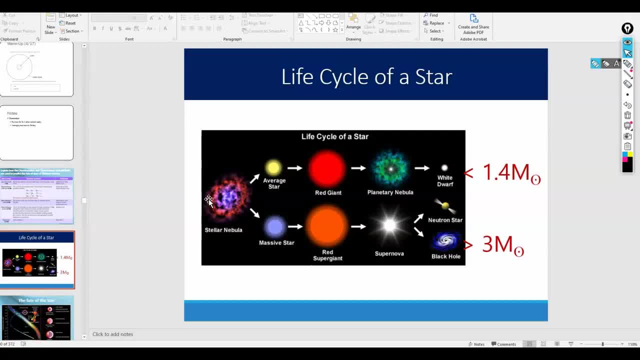 So, in other words, what we've been talking about so far in this video is basically like the top part Of this cycle, that's what's going to happen to our sun. So now it's going to. let now let's talk about what's going to happen to more massive stars and you can kind of see what's going to happen from the start. 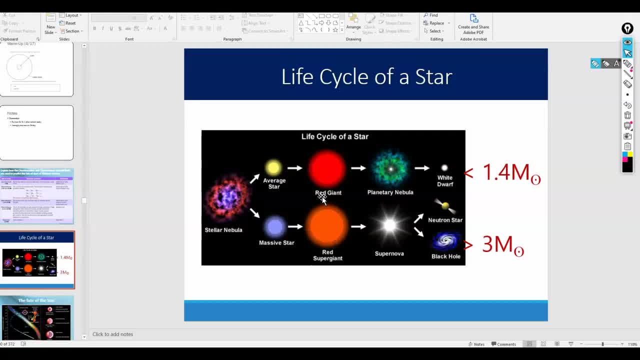 But basically, more massive stars are, rather than ending up as red giants, are going to end up as what's called red supergiants, and they're going to have so much mass that at the end of their life they're going to collapse with so much energy. 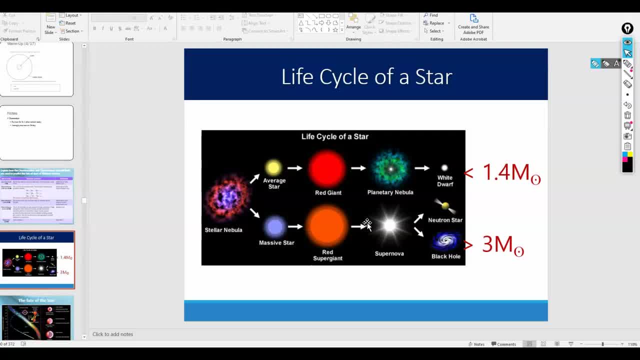 It's basically going to cause a giant explosion And that's what's called A supernova, and the result of the supernova kind of depends on the mass of the remaining core. OK, either it could end up as a neutron star or, if there's just so much mass, it's going to end up as what's called a black hole. 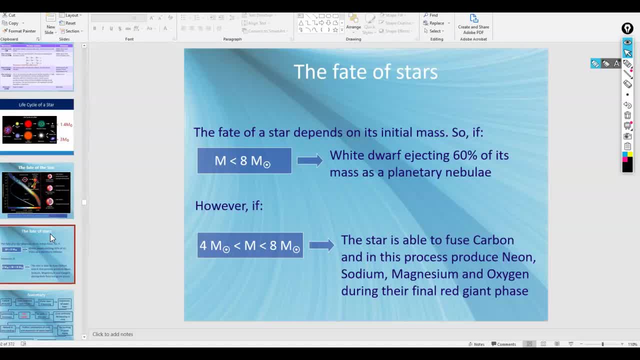 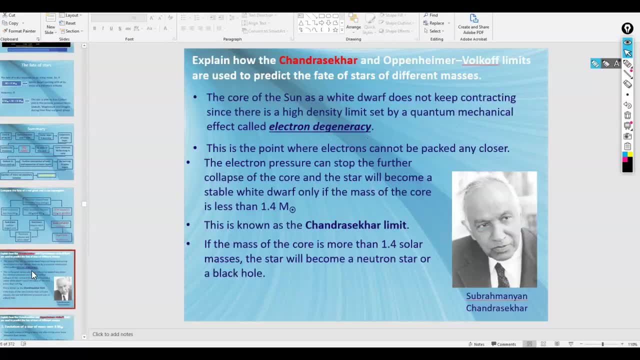 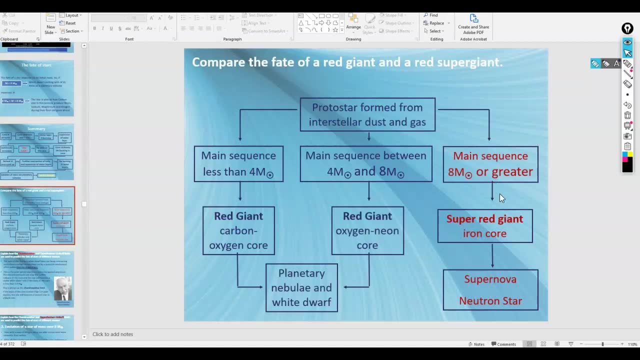 OK, so let's talk more about those other possibilities. Um see, we already talked about the planetary nebula, white dwarf possibility, Um, and this chart kind of shows you another way of what I just kind of talked about: how, um. 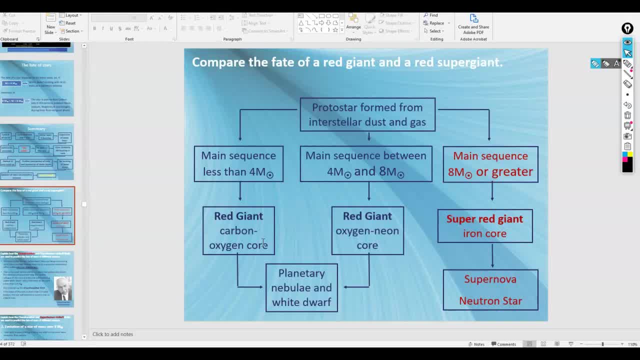 before we were talking about, like normal main sequence stars like our sun that are just going to become a red giant and then a planetary nebula and white dwarf main sequencers with a mass greater than eight solar masses are going to go supernova and either form a black hole or a neutron star. 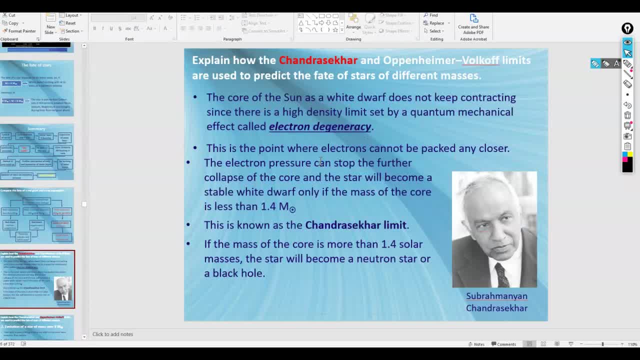 Now, as far as the whole like white door versus neutron star, like why do some stars end up as white door And some some end up as neutron stars, that has to do with something called electron degeneracy, which basically has to do with how close electrons can be packed together. 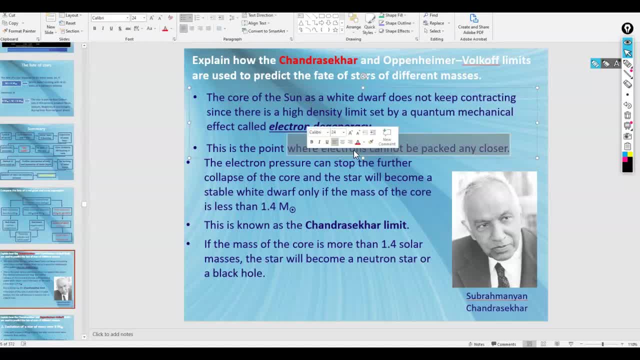 So if you have a um, if you have a white dwarf, um, white dwarfs are pretty dense, OK, but at some point, um, as you get bigger and bigger and bigger white dwarfs, you get more mass and you have this like greater pressure pushing everything together. 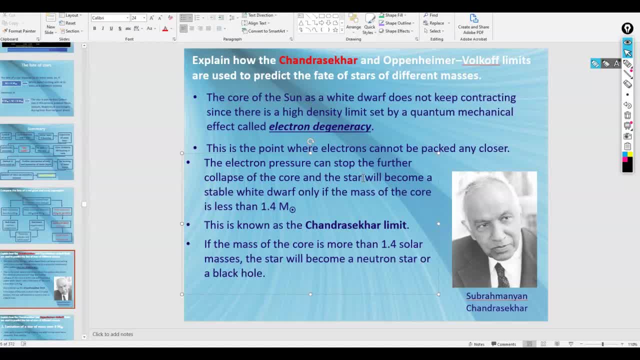 But the issue is there's a limit to how close you can press electrons Together, um, which means that there is a limit on what is the biggest possible white dwarf, And that limit is what's called the Chandra Saker limit. If the mass the core is more than 1.4 solar masses, then you can't get a white dwarf anymore. 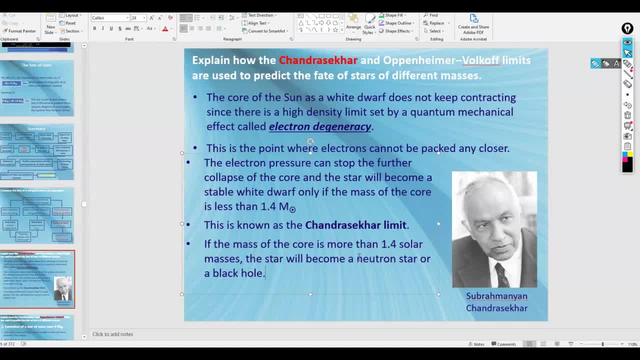 Basically, in that case, you have so much mass you're going to end up as either a neutron star or as a black hole, And so there is an upper limit on what is the biggest possible white dwarf, the biggest possible white dwarf. 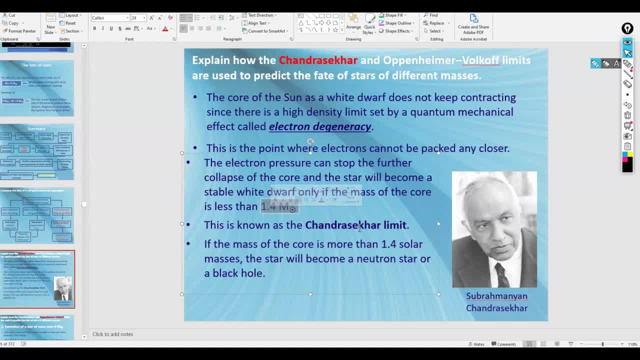 And that would end up with a mass of 1.4 solar masses. If you're confused by by that, that number um, by the way, why is it 1.4?? Because, before I was talking, I like 8 solar masses. 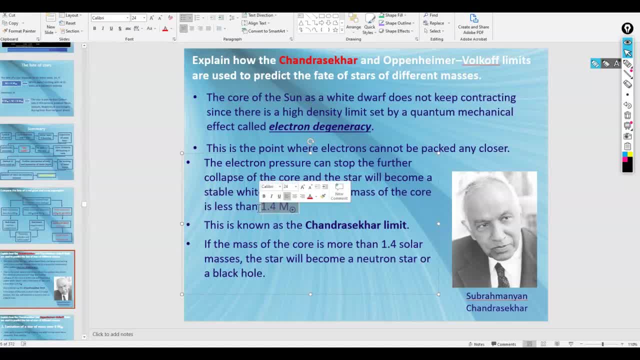 This is only the mass of the core. So remember, the core is only like a very small part of the star. So this is saying: after, after all of the, the outside shell of the star like puffs off into space and leaves behind only the tiny core. 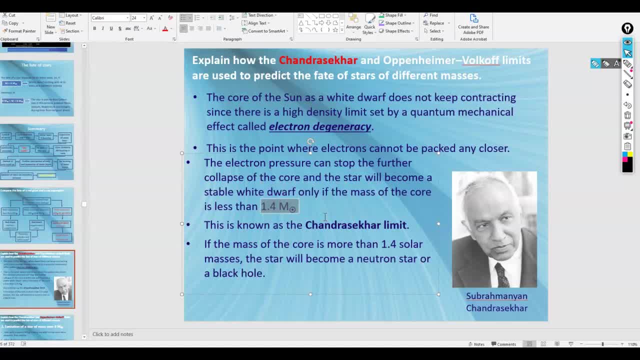 If that tiny core is bigger than 1.4 solar masses, Or in other words, if the entire star to begin with was bigger than 8 solar masses, then that's when you you don't have a white dwarf anymore. That's when you have either a neutron star or a black hole. 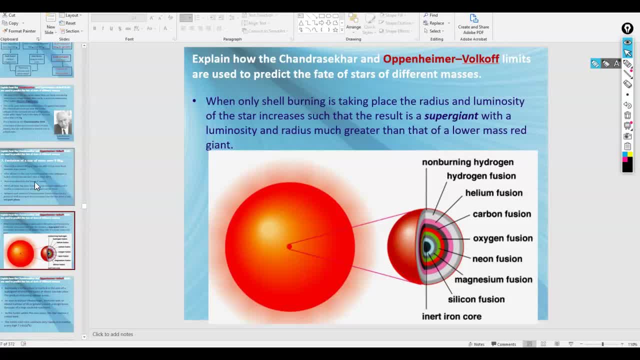 Alright, so let's see. um, I'm going to skip past some of this. This is basically talking about stars that are um bigger and so end up as super giants rather than red giants, But you still end up with these shells of different elements because, basically, that that whole process of fusion stopping and then gravity causing contraction and then setting off more fusion, basically that keeps going and going and going in in like super massive stars. 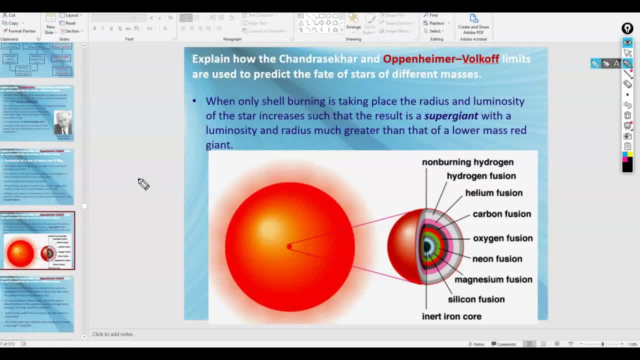 Now there is a limit to the elements that can be formed inside a star, because we've talked about this in the past unit. there's something called the binding energy per nucleon graph. The peak of the graph is something kind of like this and the peak of the graph is like iron 56, and so at some point you can't get past this point on the graph because that that element is like one of the most stable elements. 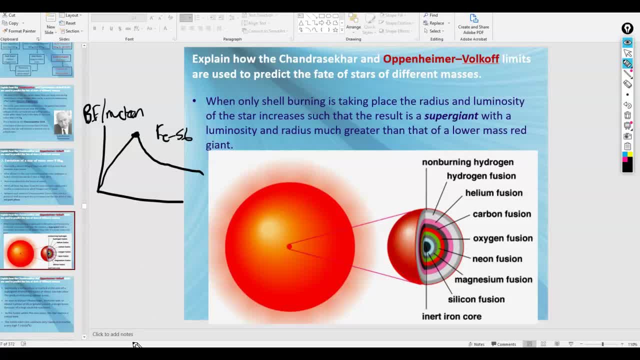 And so it's. it's not formed um naturally through nuclear fusion anymore, And so even the, the biggest super giants can't fuse elements past iron, uh inside their core. And by the way, at at this point you might ask: well, how do we get elements past iron? 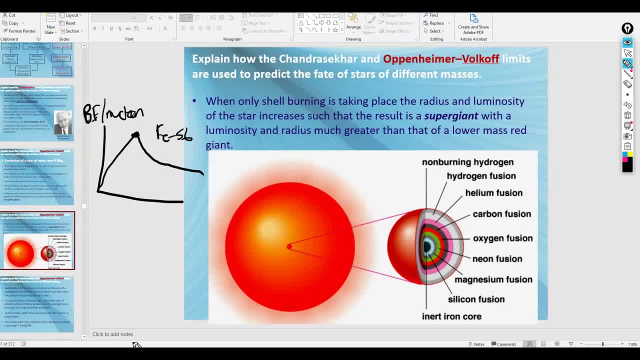 If it's not possible for them to be formed inside stars. elements past iron on the periodic table are actually formed from supernovas. Okay, because in a supernova the explosion produces so much energy it can produce those heavier elements Okay, which, if you think about it, it's kind of cool. 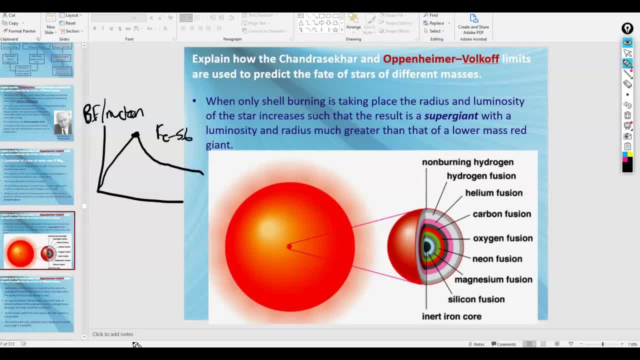 That means every element past iron on the periodic table that we see on earth at some point must have come from another star that lived and died like a long time ago, like billions of years ago, Because those are the only ways that we know, The only way like heavier elements, um can form in the universe. 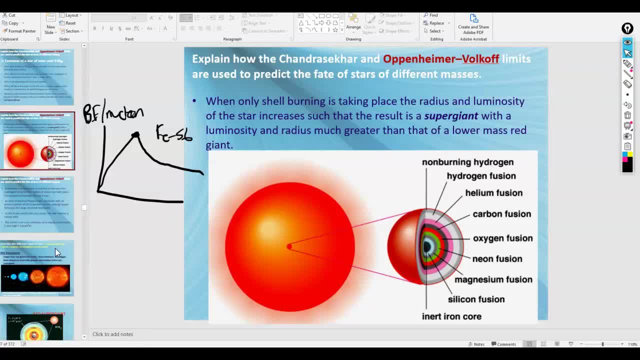 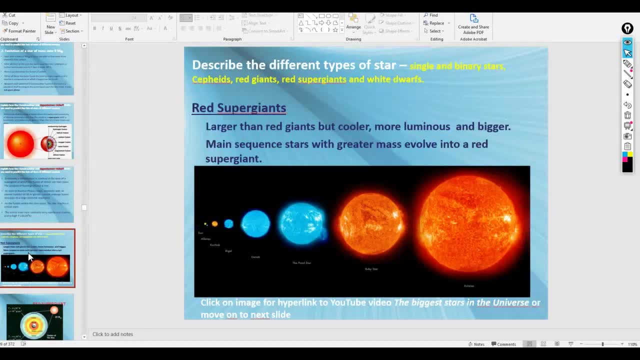 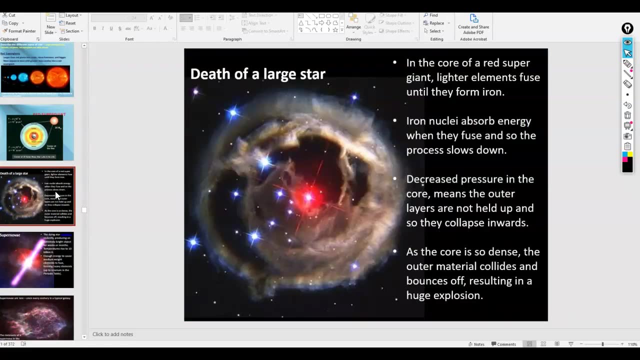 So we, we are all literally like stardust essentially, But anyway, um, let's see, I talked about that red super giants, different layers of elements, talked about that before. Okay, so the death of a large star. 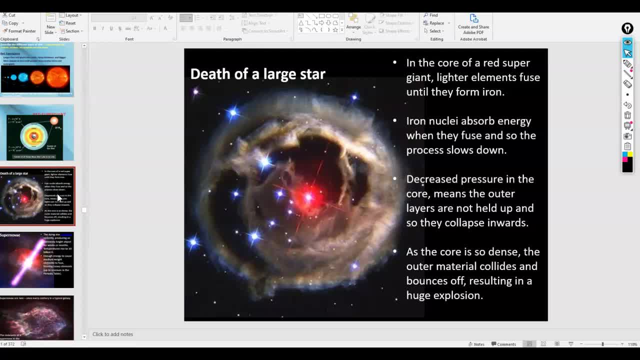 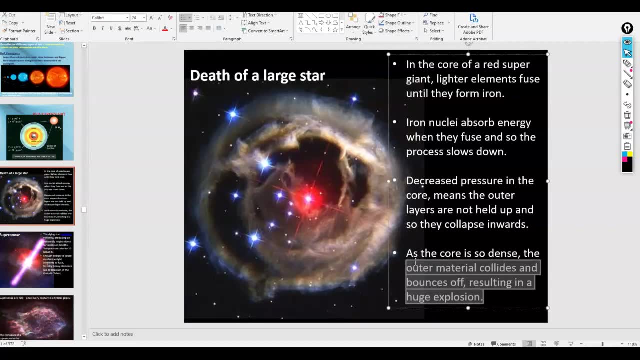 So once you get to the iron stage you can't form any heavier elements, And so eventually the um, the fusion, is going to stop, And so that means all that gravity is going to kind of collapse, everything in towards the core And it's going to result in a giant explosion, because all that inward pressure is basically going to bounce off the core. 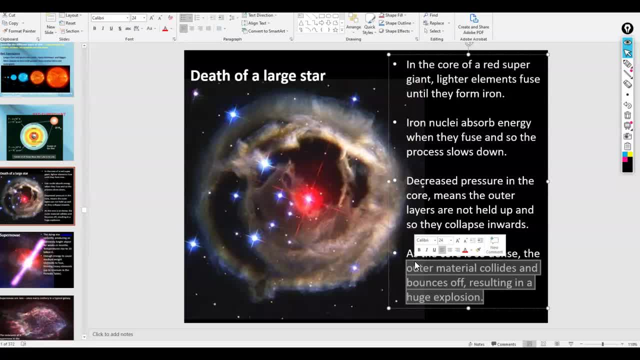 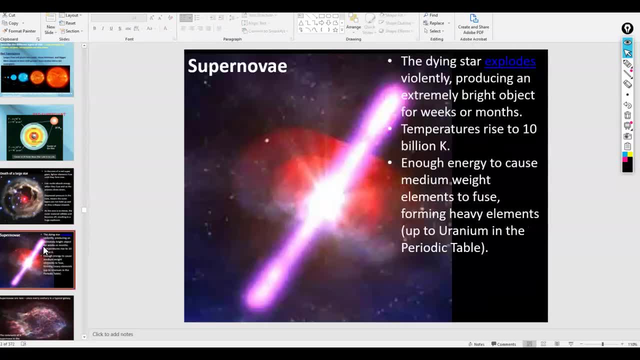 And then it can't, it can't go in anymore. so the energy is going to produce a shockwave- Sorry, it's going to produce a shockwave that goes out and that is the supernova, And it is basically like a ginormous explosion. 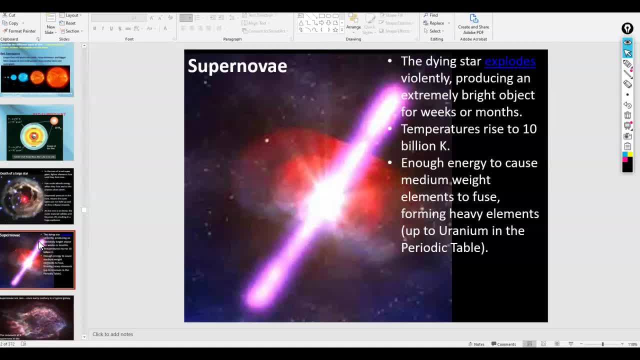 Um, in fact we can actually see it If there's a star close enough to the Earth. we can actually see the supernova from um, from Earth in the sky, And if it's close enough, we can even see it for for like days or weeks after the star's uh death. 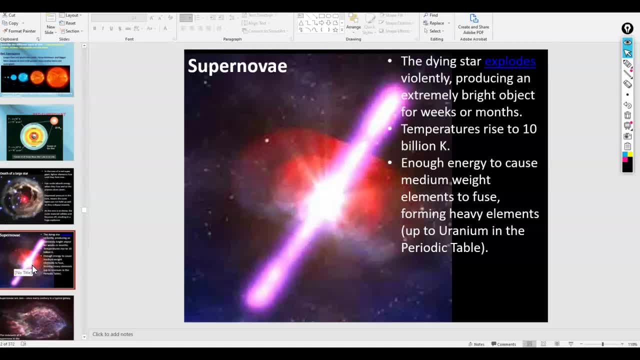 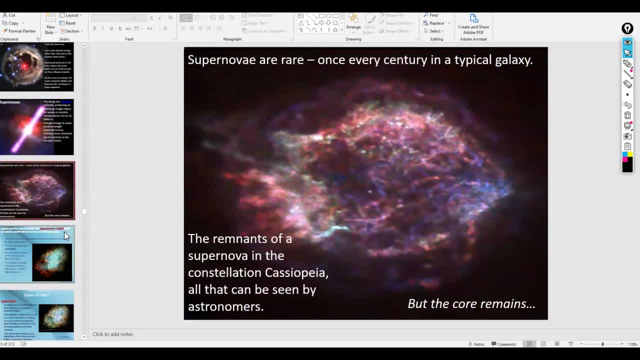 Which is really cool, And during that giant explosion, that's where you form the heavier elements all the way up to uranium on the periodic table. Okay, and so these are not super um common, But when they do happen, if they happen close enough to the Earth, even though they're, they could be like. 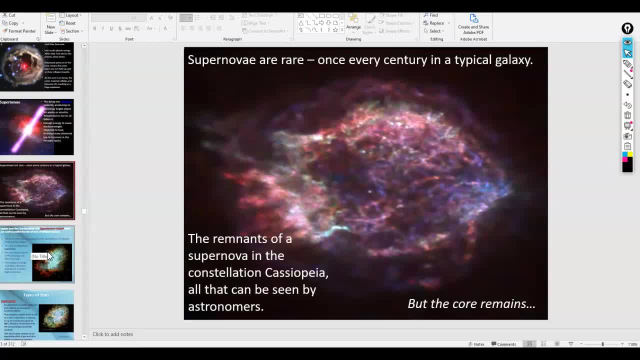 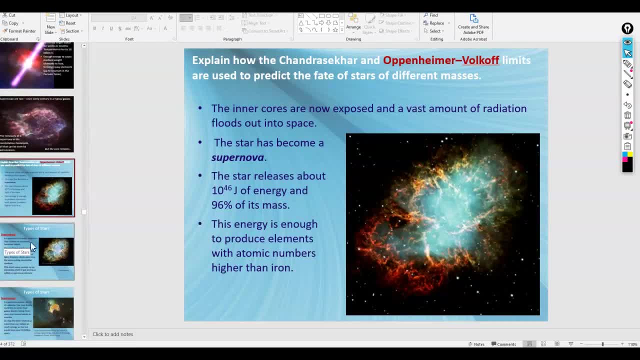 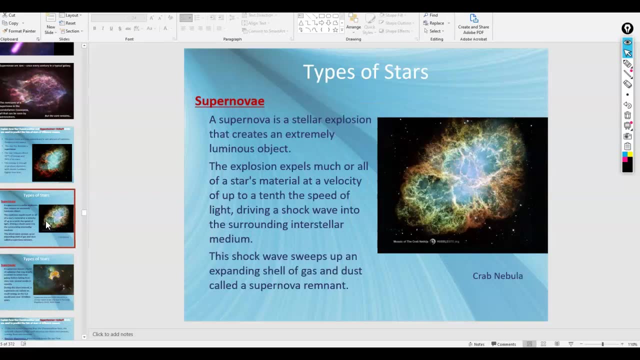 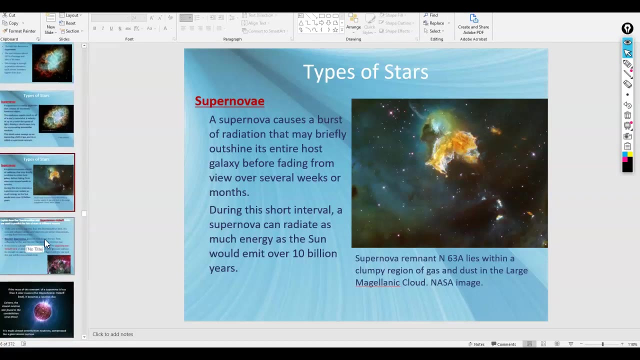 thousands of light years away. they're just so big and massive that they're even visible that far away from Earth, Which is pretty cool. Okay so, supernova, giant explosion Just going to click through these slides. Okay so, during this short interval of the supernova, 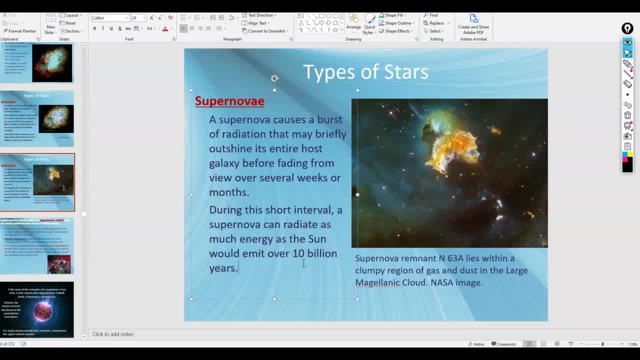 it can radiate as much energy as our sun would emit over 10 billion years. Okay, so so think about that, Think. think about like power as energy over time. So think about how powerful that explosion is if if you're taking all the energy that our sun puts out over its entire lifetime. 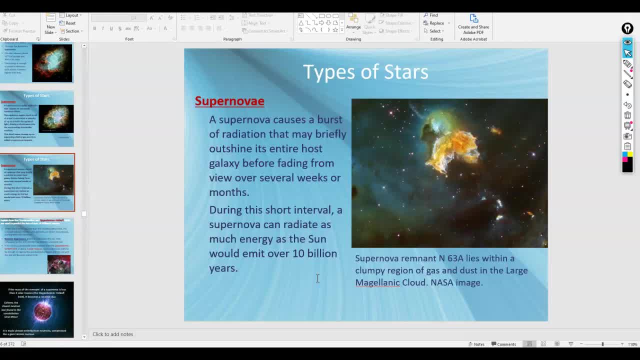 spread out over just like like a few weeks. It's a massive amount of energy. Okay, so I'm going to go ahead and stop this video here. Um, we've talked about what a supernova is and the energy produced.